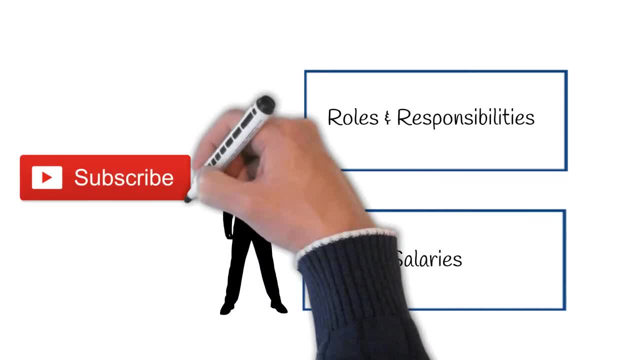 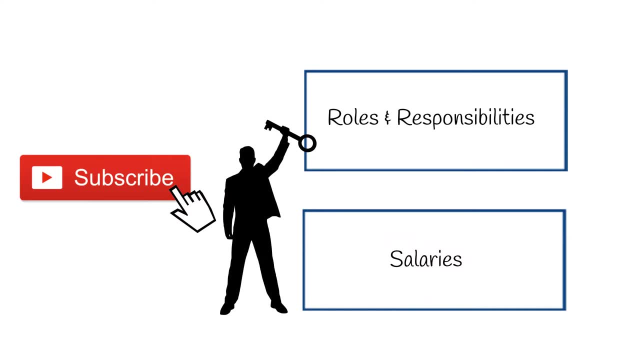 if you're enjoying these videos or have found them useful in any way, please be sure to subscribe and hit the notification icon to get alerts when we upload new content every Wednesday. Also, this week's video has been requested by you guys- Steve, Teddy and Kev. 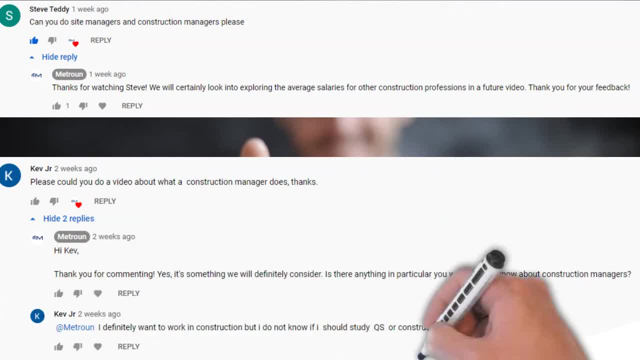 Jr both requested a video on construction managers, So if you'd like us to cover any topics, please write in the comments section below. So the best way to start this video is to subscribe to our channel, If you'd like to. 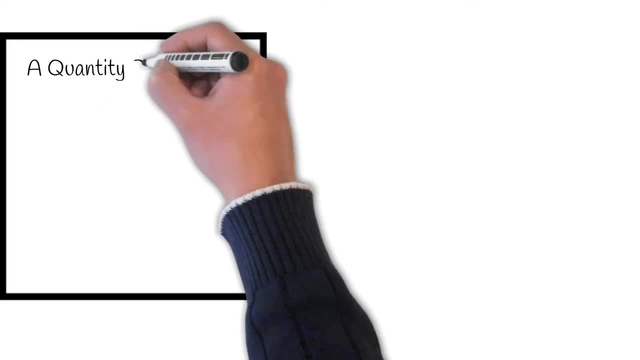 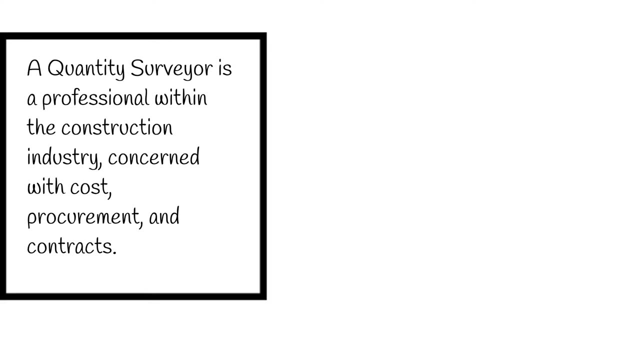 is by giving you a definition of the roles. A quantity surveyor is a professional within the construction industry concerned with cost procurement and contracts. To make it even more simple, the main reason a company would hire a quantity surveyor is to accurately. 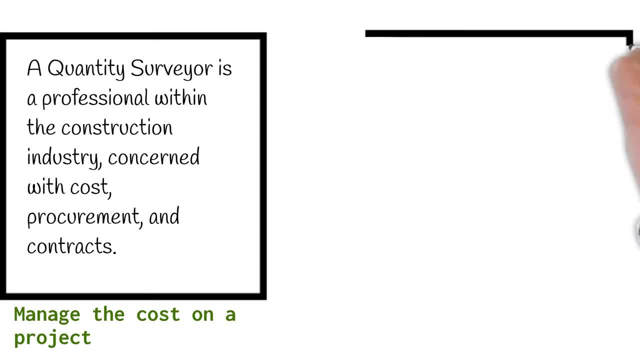 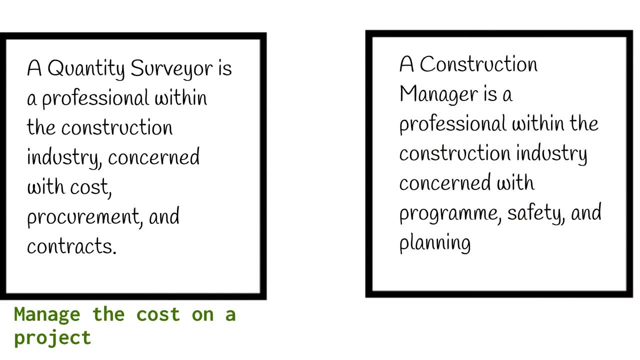 manage the cost on a project. A construction manager, sometimes referred to as a project manager or site manager, is a professional within the construction industry concerned with program safety and planning. Simply put, a company would hire a construction manager to safely oversee a project and manage the cost of a project. A construction manager- 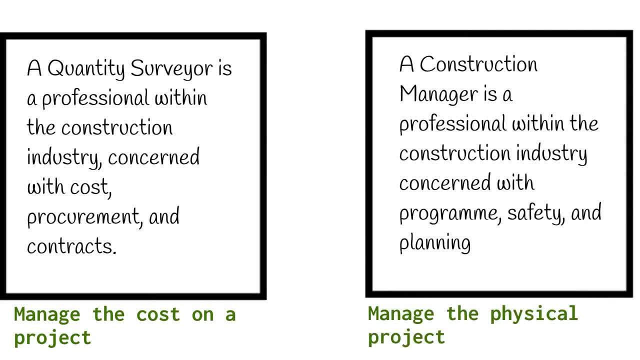 is a professional within the construction industry concerned with cost procurement insurance completed on time and on budget. So here's a first difference: A QS is focused on the cost and value of a project and a construction manager is focused on the program. 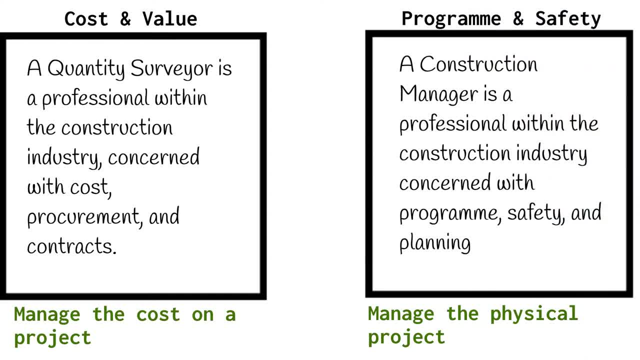 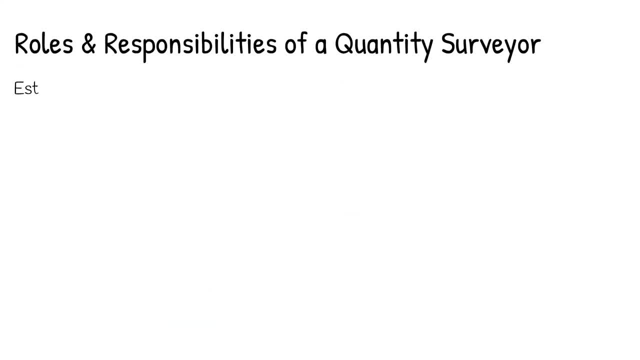 and safety of a project. Now you're probably wondering what a day in the life of a QS and construction manager is like. also, A normal day for a quantity surveyor may include estimating or forecasting the cost of labour plant material required for a project preparing. 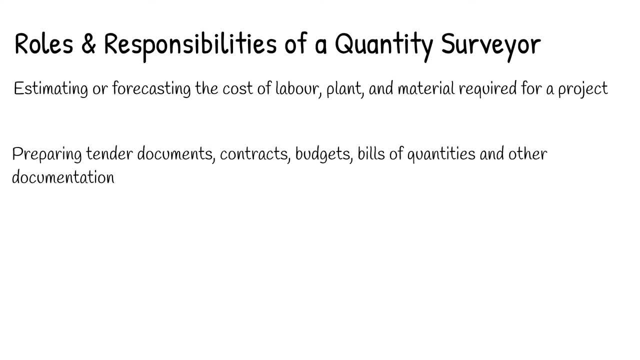 tender documents, contracts, budgets, bill of quantities and the like. So if you're going to be doing a mon, Knight'snejård or Wow coming in 2020, you don't necessarily require that one Catch on date there: monthly time, years, points of chance, etc. 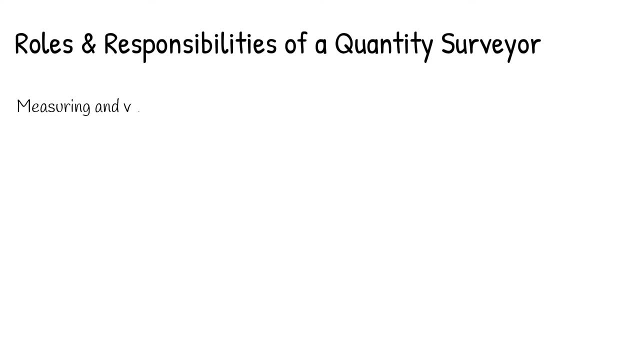 contractors who work on the construction of a project, Measuring and valuing the work completed on site, issuing payments to subcontractors, liaising with the client and other construction professionals, such as site managers, project managers and site engineers, and selecting and. 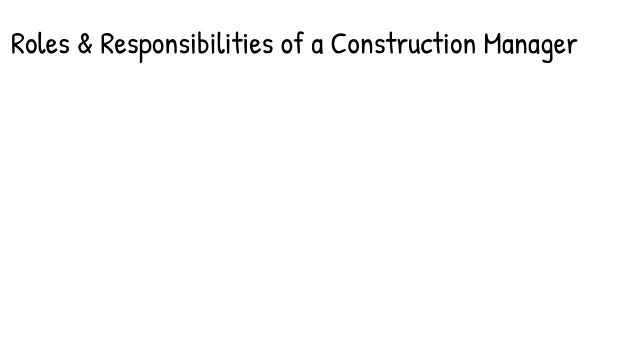 sourcing construction materials. A normal day for a construction manager may include planning and coordinating a project from start to finish, including organising the schedule of work, hiring and managing staff for a project. managing the construction site on a day-to-day basis, including supervising the labour force, monitoring subcontractors, checking materials, inspecting work.